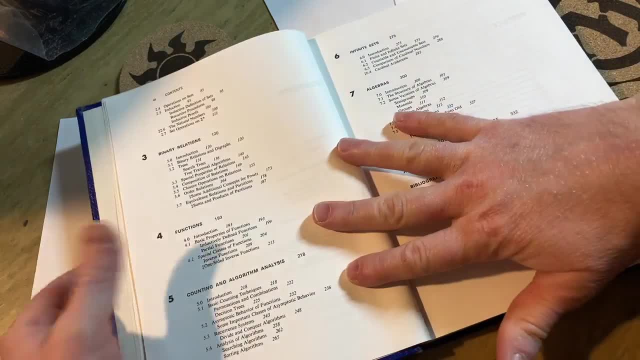 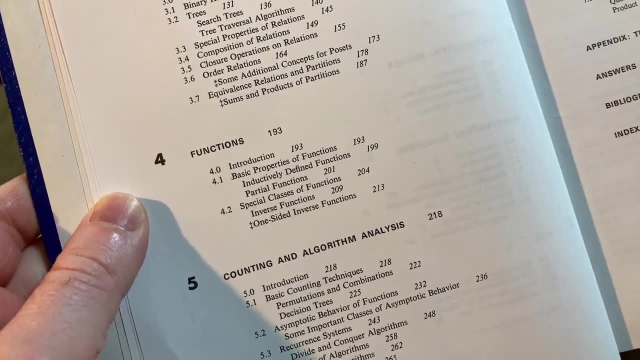 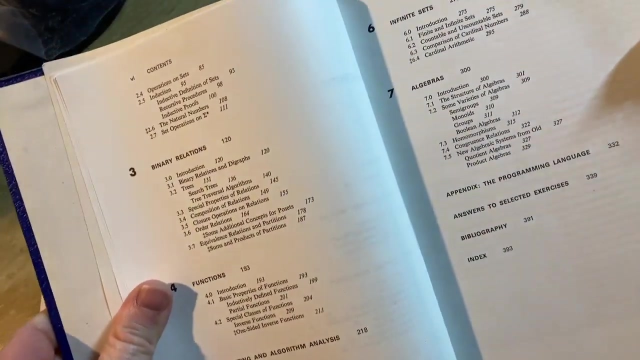 And we'll take a look at it just so you can see how hard it actually is and what you think. Binary Relations, Functions, Counting and Algorithm Analysis. We have Infinite Sets and Algebras, And it does have answers to selected exercises in the back of the book, which is quite nice. 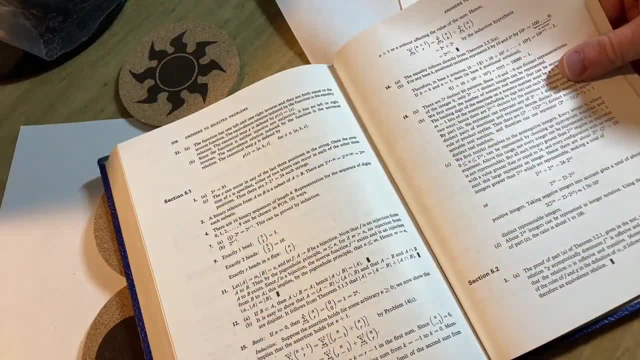 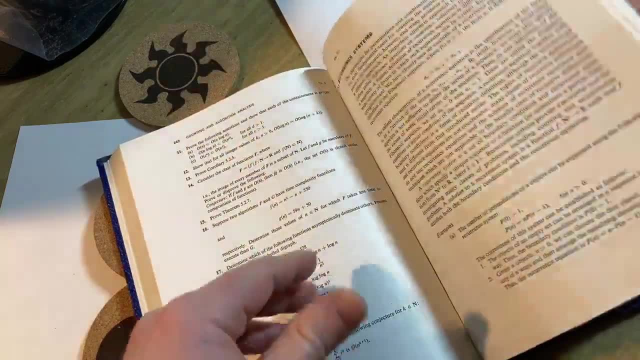 Most of these books do. This is a fairly modern book, even though it's older. The style is nice, It's a nice, clean book, Clean book. So you do have answers to some of the problems And he actually works out the answers, as you can see. 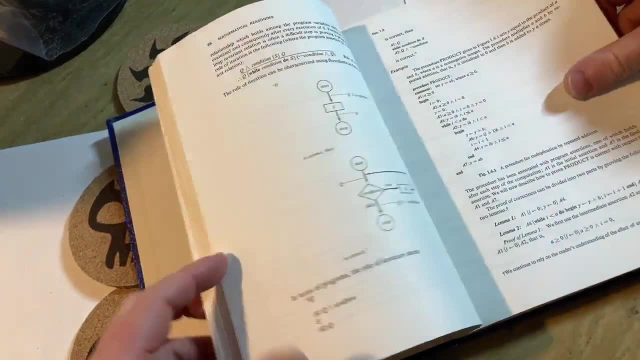 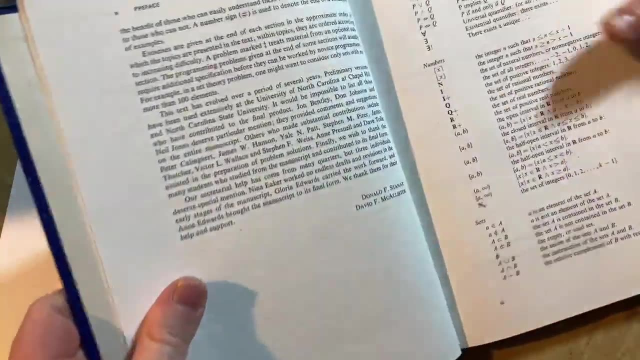 Even the proofs When the answer is given, right, As the answer is not always given. Let's go to that beginning, just because I told you I would show you Here. it talks about all the symbols. It gives you all the notation that you see. 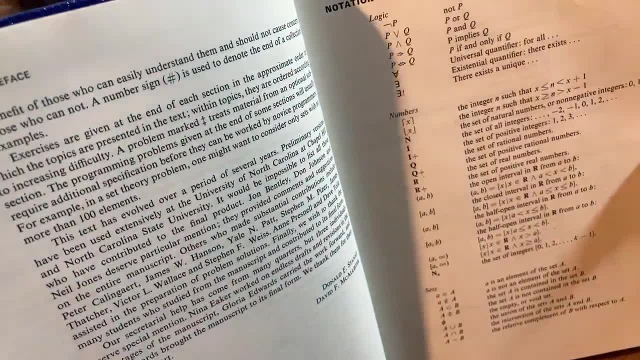 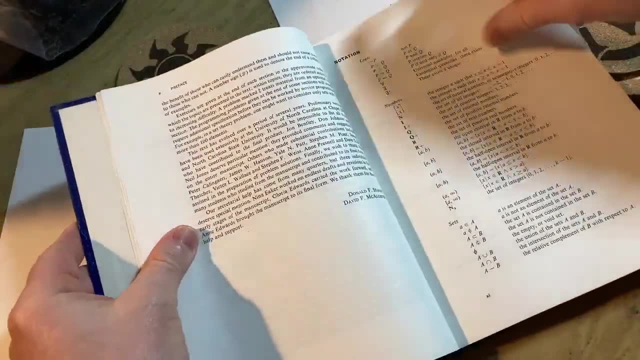 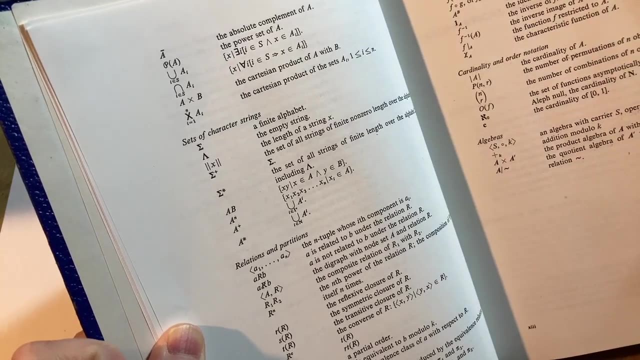 You have all those logic symbols. You learn those when you study logic And you can learn those in this book: Number symbols, Numbers Sets, Even more symbols, right, All kinds of symbols. So that's kind of nice. So if you are reading the book or you just open the book as a reference, you're like 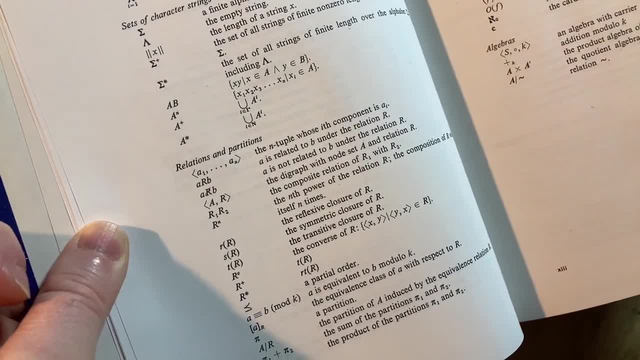 oh, what does that mean? If it's not clear in the section- perhaps it's defined in a previous section or something and you don't know where to find the definition- you can go here and this tells you what the symbols are. 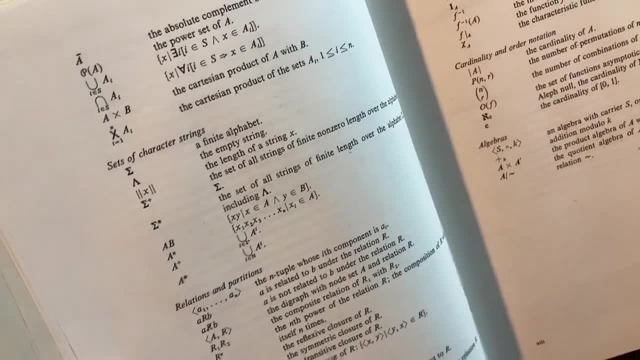 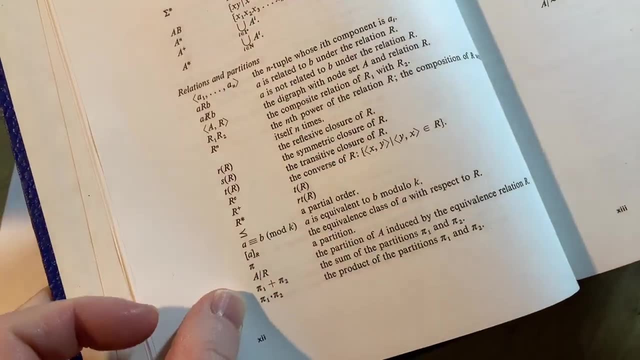 So the more math you know, the more you start to learn all these symbols. Eventually you know what all of these symbols are, And if you don't know you can just read it, For example, like here: Like pi sub 1 plus pi sub 2.. 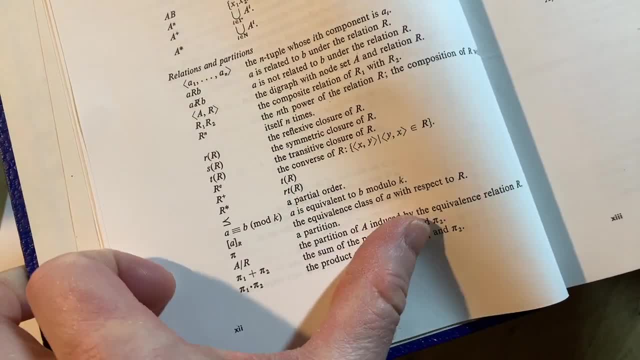 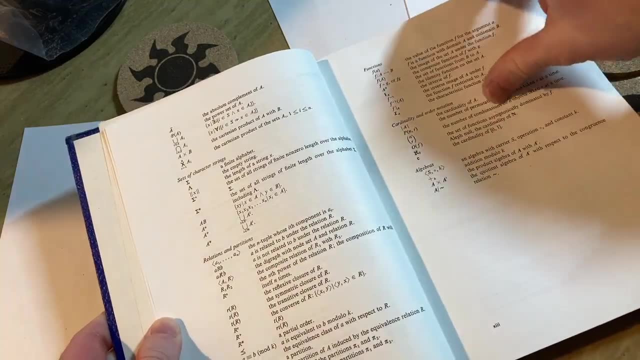 What does that mean? That could mean anything, right? So here it says the sum of partitions pi sub 1 and pi sub 2.. Okay, All right, Stuff like that, You know. you might not. Even if you already know math, it's still beneficial because you might not know exactly what they mean in that particular case. 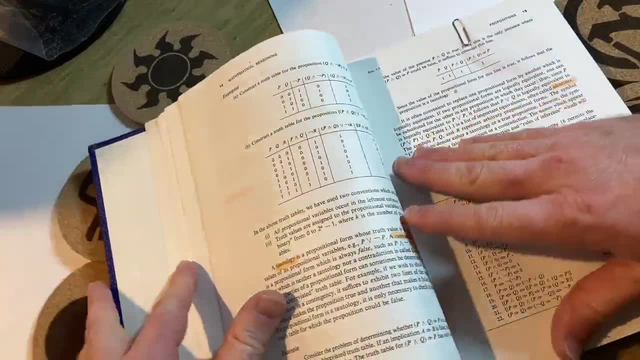 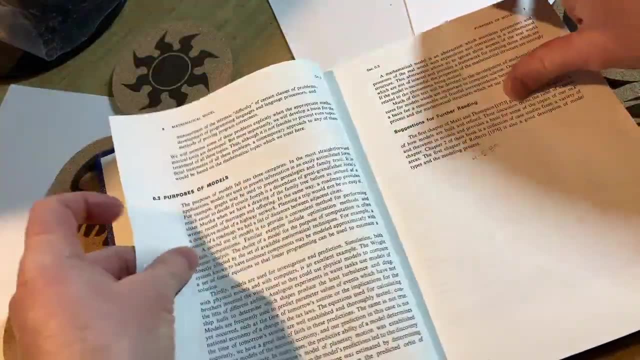 This is chapter 0. It's on mathematical models. Let's go to chapter 1 so I can show you how it starts, So you can make a decision as to whether or not you think it's a good book. And discrete math is hard. 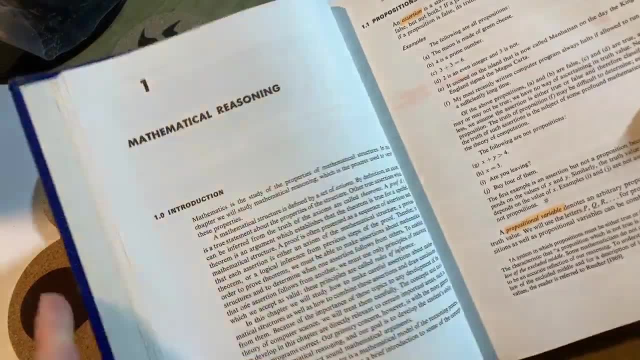 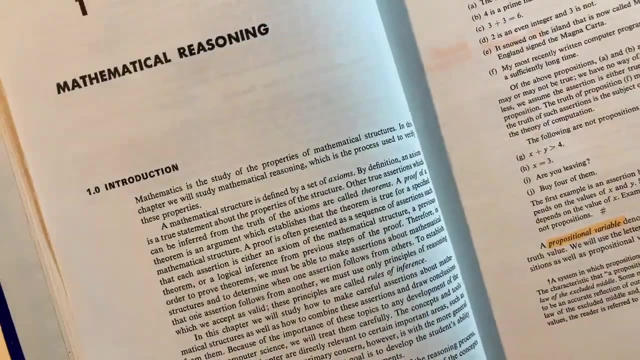 When you take discrete math you know you usually have a book for the course. In my experience it's always a pretty hard book because most discrete math books are pretty hard. So having lots of discrete math books I think is good because it makes it easier to learn the subject. 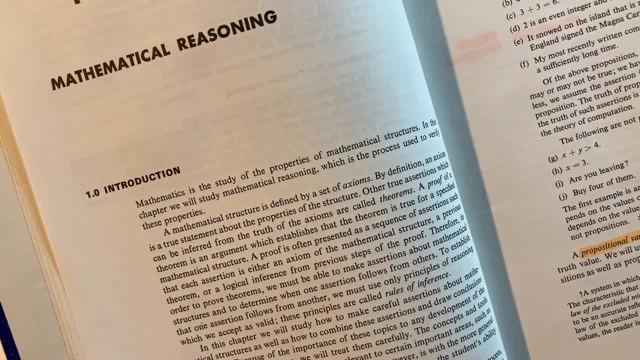 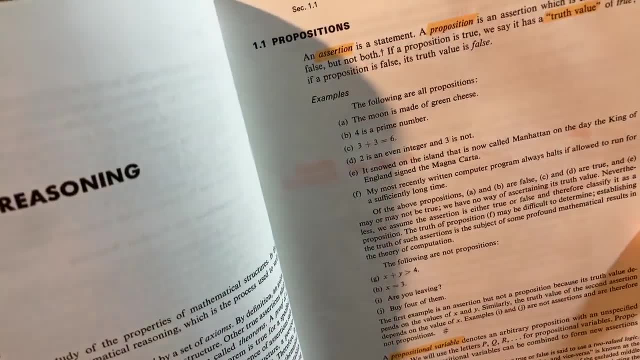 It says: mathematics is the study of the properties of mathematical structures. In this chapter, we will study mathematical reasoning, which is the process used to verify these properties. right, So yeah, Propositions: An assertion is a statement. A proposition is an assertion, which is either true or false, but not both. 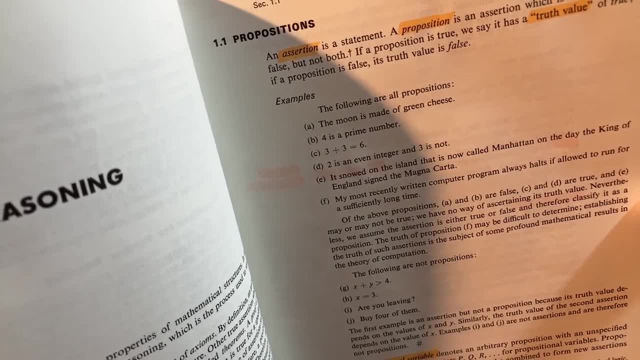 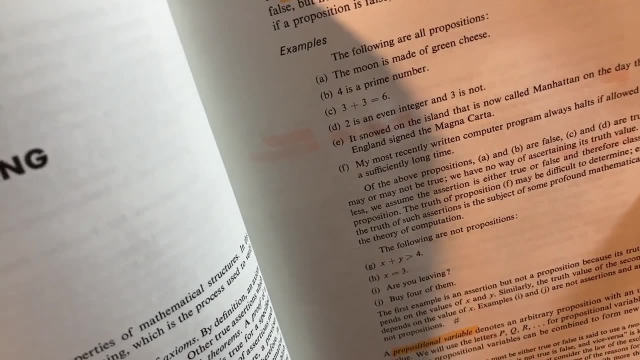 Proposition is true, We say it has a truth. It has a value of true. If a proposition is false, its truth value is false. The following are all propositions: The moon is made of green cheese. Four is a prime number, right. 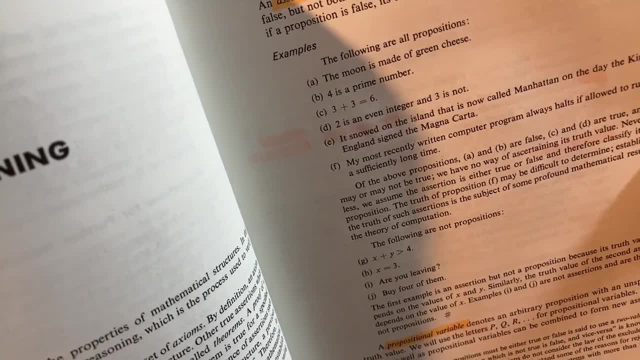 Some of them are true. Some of them are false. right Four is not a prime number. right A: the moon is made of green cheese. That would be true. No, I'm kidding, It's not made of green cheese. 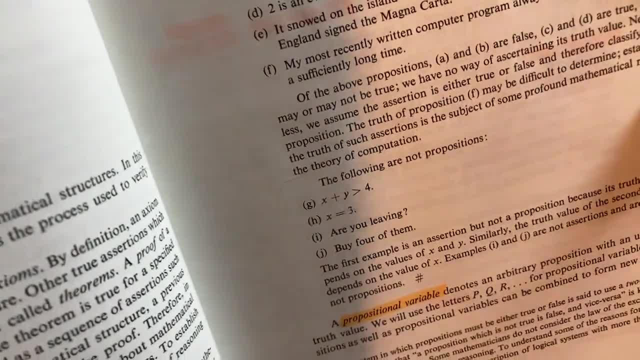 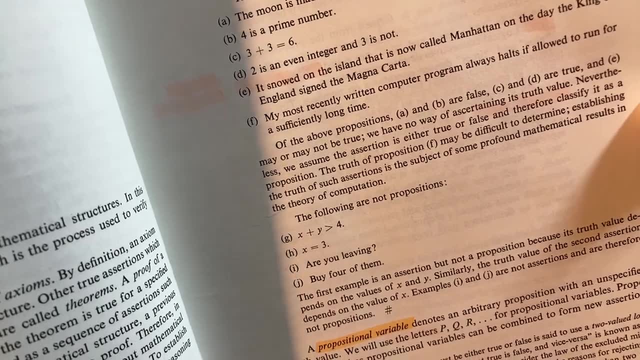 But I mean so everything is a true or false statement, And then here's things that are not propositions. Okay, The first example is an assertion, but not a proposition, because its truth value depends on the values of X and Y. 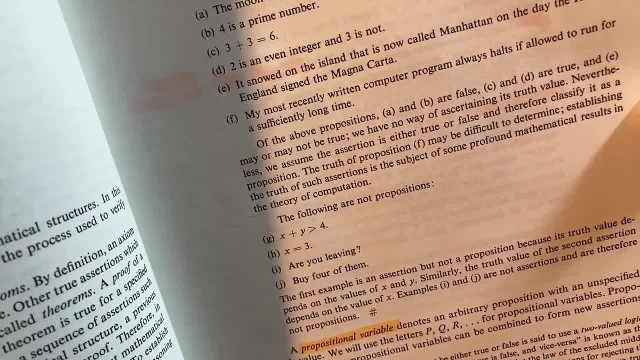 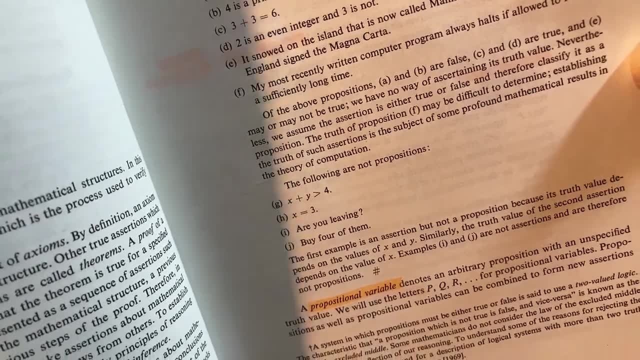 Similarly, the truth value of the second assertion depends on the value of X. right. Examples I and J are not assertions and are therefore not propositions. Are you leaving? Buy four of them, right? That's not true or false. Interesting right. 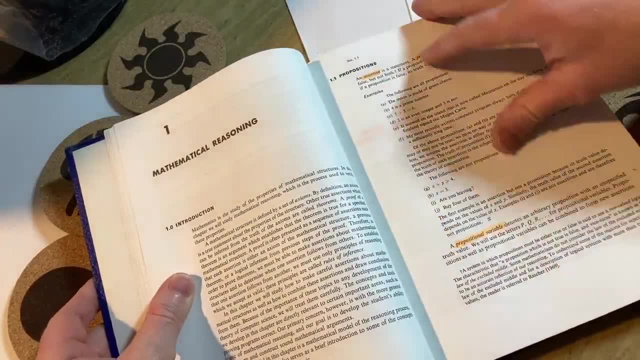 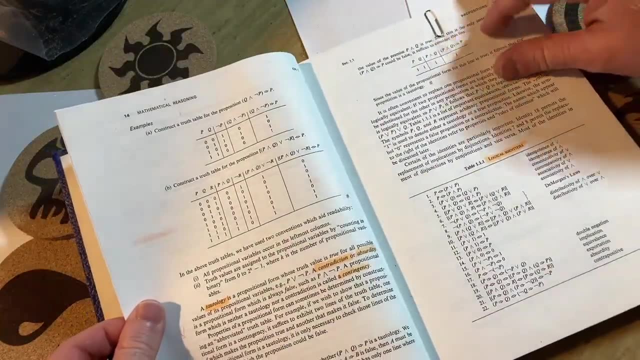 So it explains everything quite well And it explains why those are not propositions, right? I thought that was a pretty good explanation And you can read it and go from there. I'm going to put a paperclip in it. That was not me. 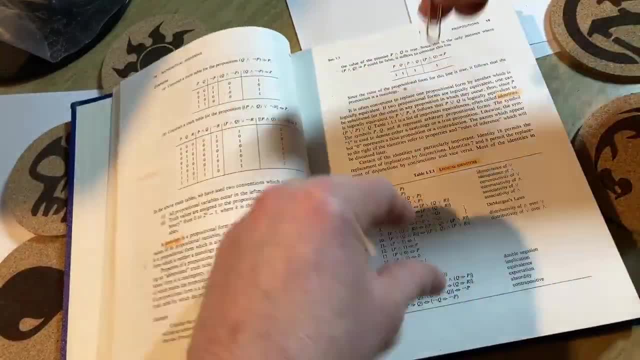 I'm going to leave it. Oh, maybe I should take it out, Oh, I don't know. Now, it's going to leave a mark. What do you do with stuff like this? I have some books that have like rusted paperclips in them. 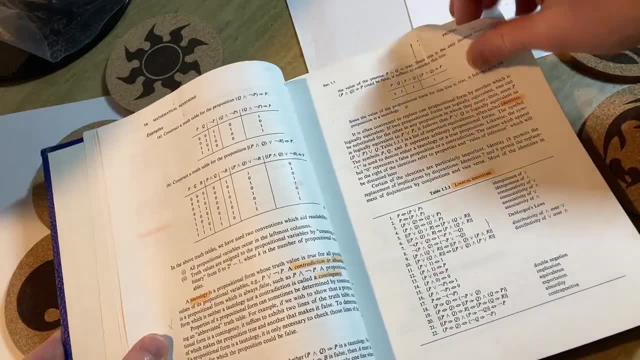 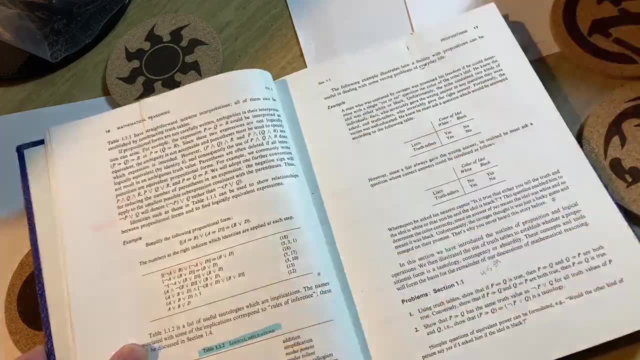 I'll just take it out Relic from the past. How old was that paperclip? Was there any other paper that it clipped in its lifetime? Interesting the highlighting and the writing in old books: right, Got some exercises. Looks like it's got quite a few exercises. 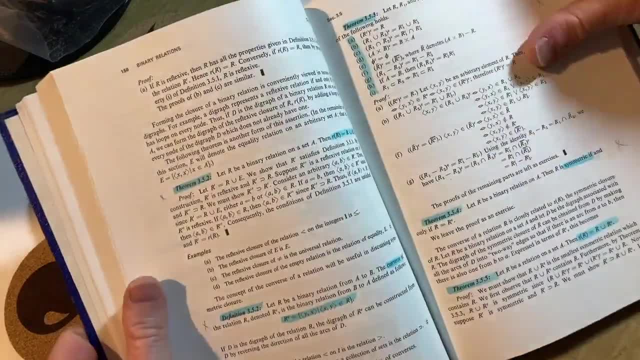 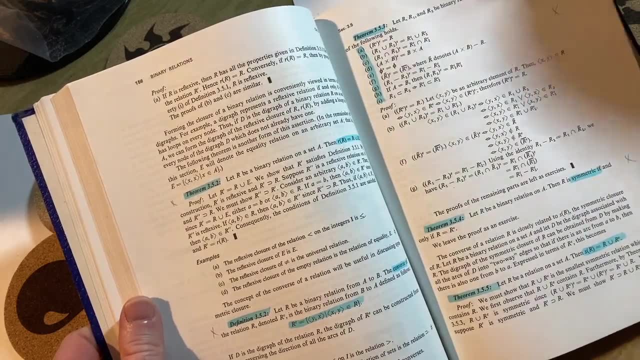 Kind of nice Jump around. It's talking about relations. Relations are really important. There's a special type of relation that's even more important. It's called an equivalence relation And you study those in a book like this. It should be somewhere here. 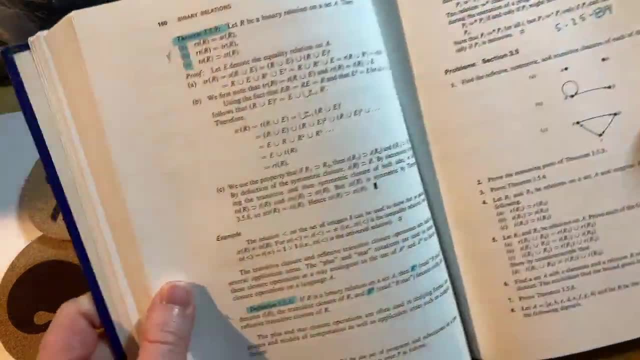 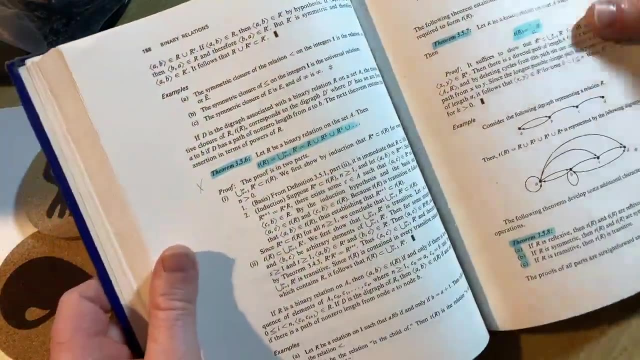 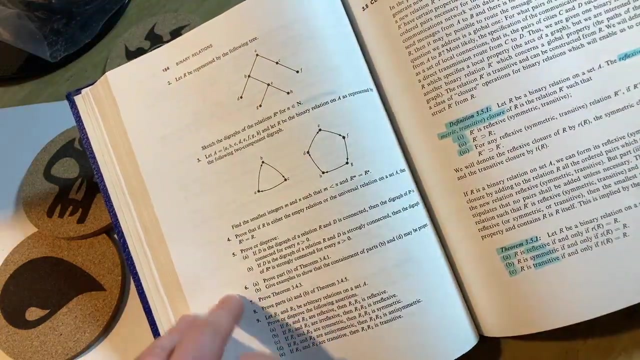 Equivalence relation. It should be here. I don't see the word equivalence relation, But here it says it's talking about reflexive, symmetric and transitive. So basically, if a relation is symmetric, reflexive and transitive, it's an equivalence relation. 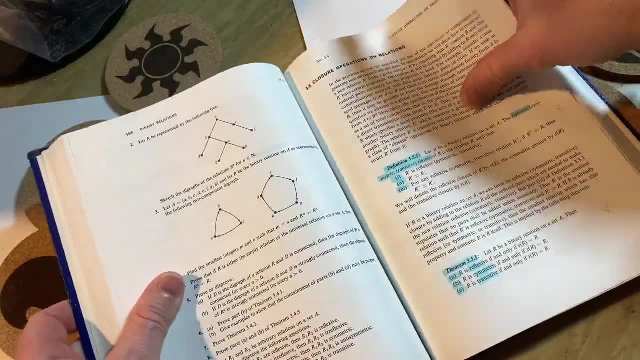 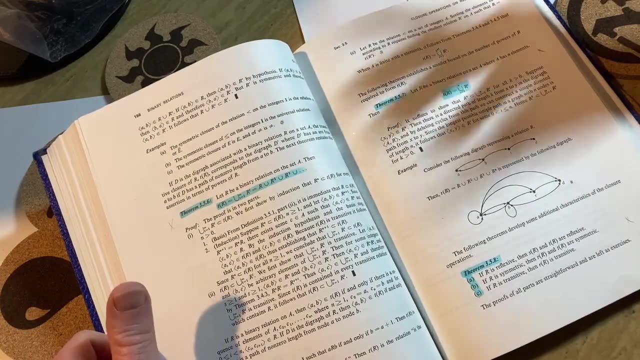 Here it talks about those things: reflexive, symmetric and transitive. Notice, there's highlighting here. That's because the person who had this book before me probably used this for a course And this is something you would cover in the course. 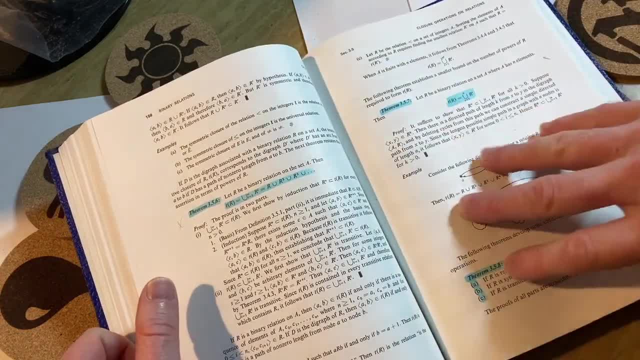 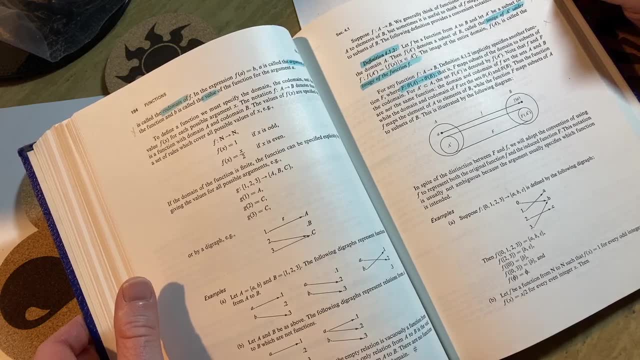 So like you could buy this or buy any book on discrete math And you could self-study so that when you take the course you're prepared. That's what I did for discrete math. I studied a lot during the course and a little bit before it too, because I had heard it was a really hard class. 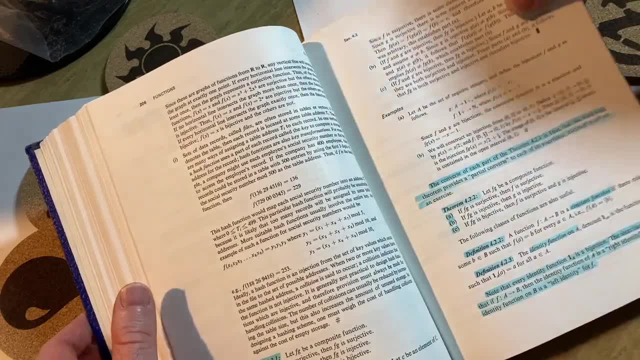 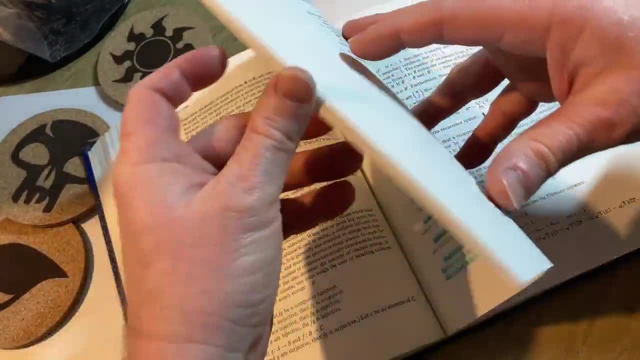 So I did really well. That was like a big victory for me. Big victory. I had the highest grade in the class And we had- I think we had- 300 students to start with. By the second test, half the class was gone. 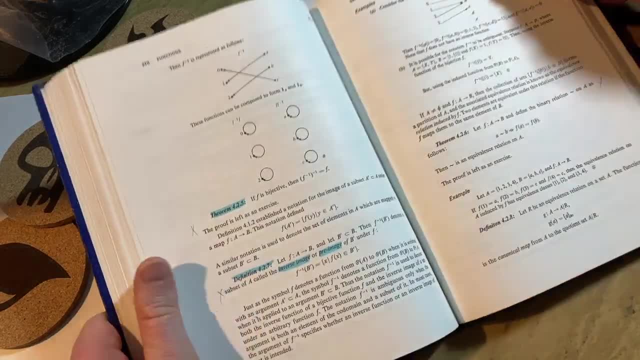 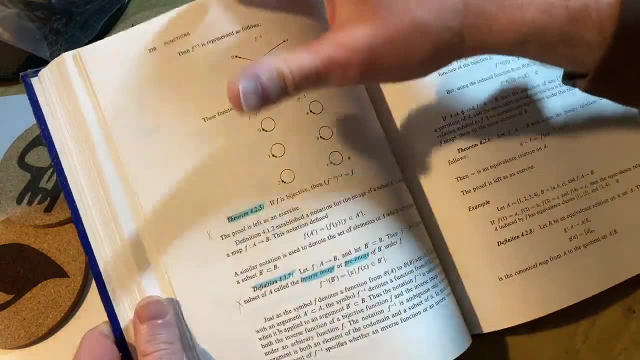 You know, it was like a massacre, like a bloodbath, And the teacher was really good. He was really really good. I thought he was awesome, But it's just the material. you know, People say books like this are tough because the topics jump. 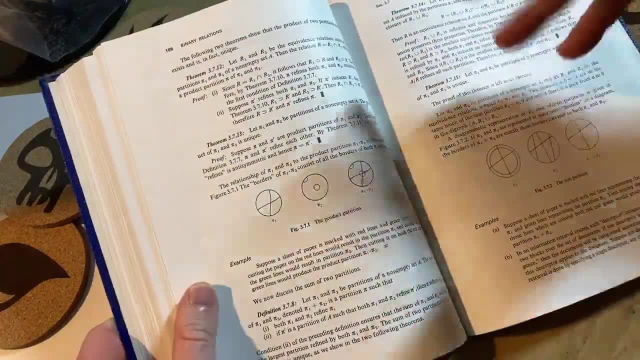 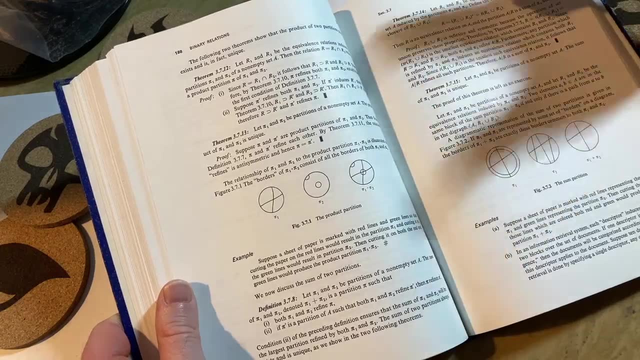 You know you're jumping from one topic to another And also it's very different from like algebra. You know, up until this point you're like: okay, algebra 1,, algebra 2, geometry, You take trig. 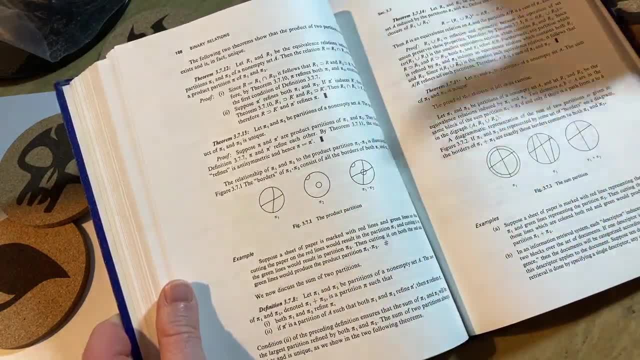 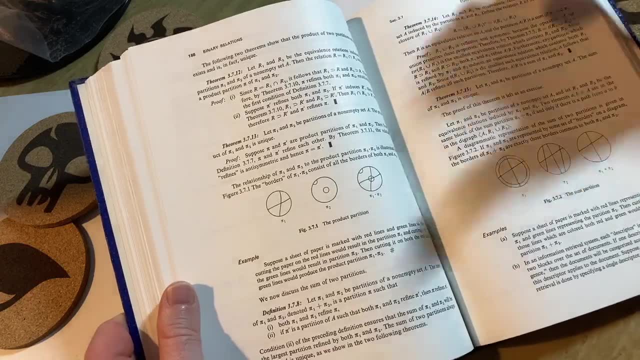 It's all algebra-based And you do like some calc 1, calc 2, maybe you know, And then all of a sudden you know maybe even calc 3 and differential equations, And then you take this. So it's just very different from that type of mathematics. 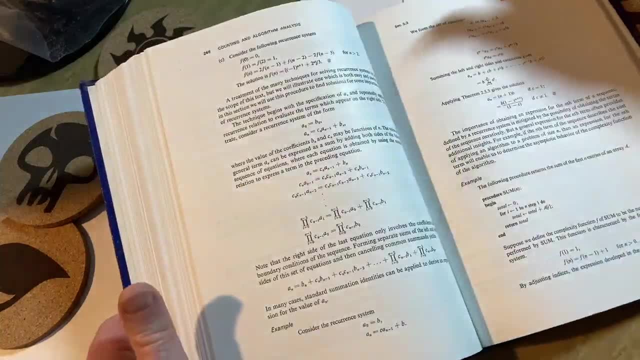 But it's a decent book. It's got good expectations, It's got good explanations, It's got good exercises And you get answers to some of the problems. I mean it's not bad, It's pretty good. I like it. 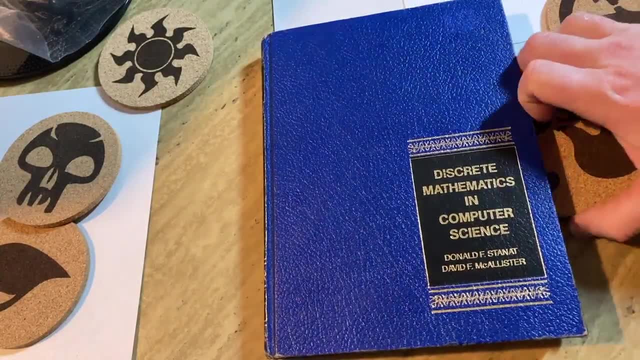 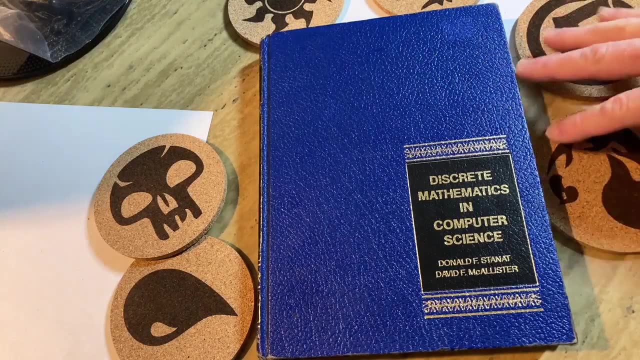 I think it's good. There's certainly other books that are harder than this one. Yeah, Easier books are usually better for learning, because if they're easy, that means you can understand them. At the same time, if they're too easy and you already know the material, they're not so good. 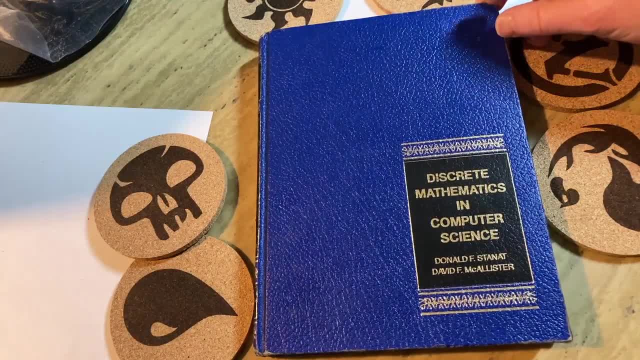 Anyways, a random video on this book. I have Greek Mathematics and Computer Science. I'll try to find it. by the way, I haven't looked, But I'll try to find it. I'll try to find it after making this video. 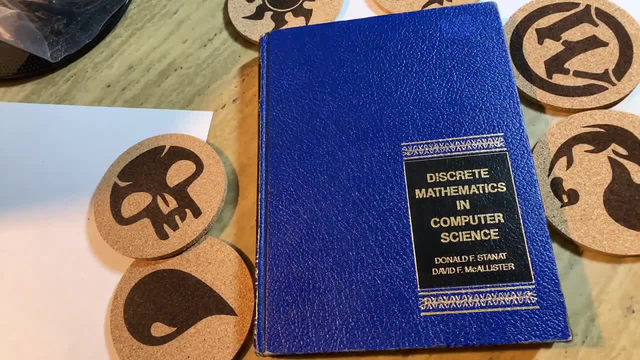 And I will post a link in the description in case you want to check it out. Until next time, good luck, Take care. 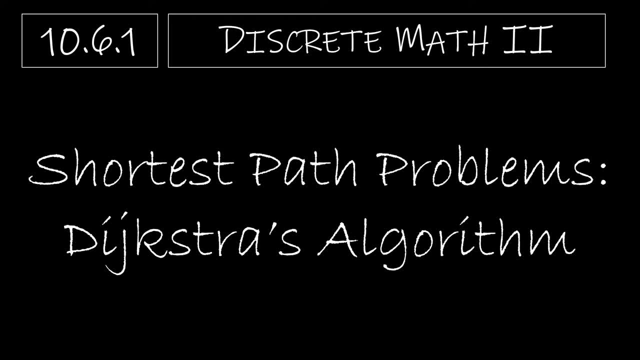 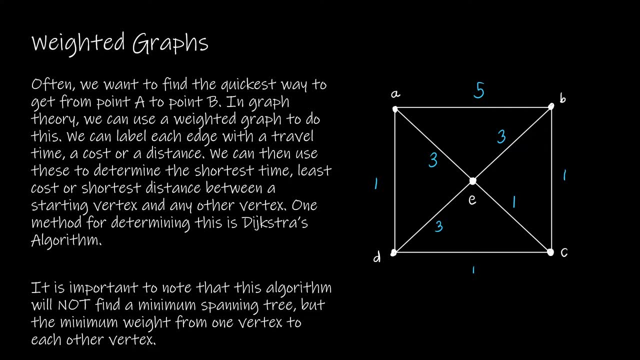 In this video we're going to take a look at shortest path problems and a way to solve them, and that way is Dijkstra's algorithm. So the way that we're going to model this is using something called a weighted graph, And in a weighted graph it can be directed or undirected, Obviously, 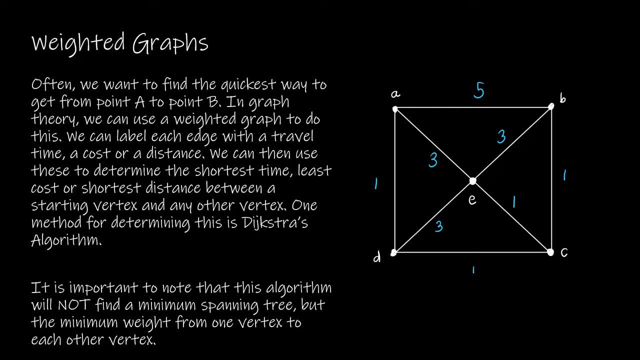 the graph model I have here is undirected And essentially we're just going to label each edge with a travel time, a travel cost, a travel distance or whatever it is that we're trying to model with that particular graph, And then we can use those to determine the shortest time or 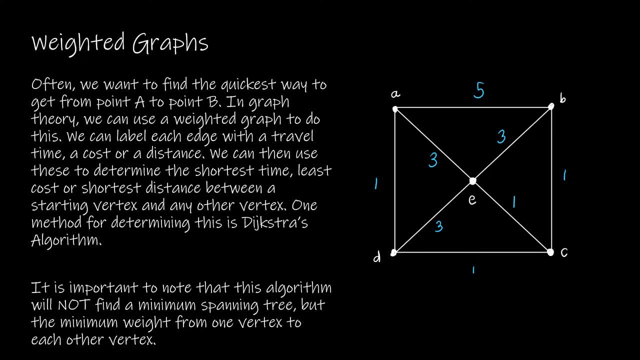 the least cost or the shortest distance between some starting vertex and any other vertex. So in our example, we are going to use vertex A as the starting vertex, And what it's going to do is it's going to find the fastest way to get to B. 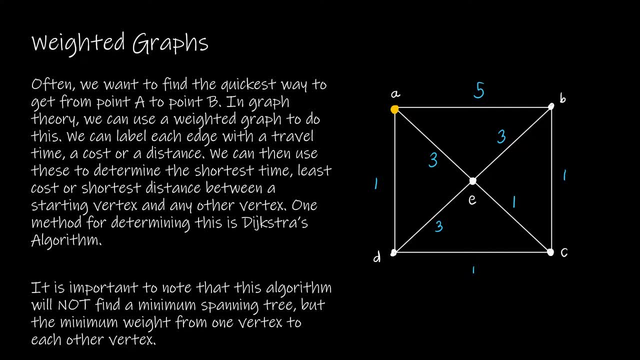 The fastest way to get to C, the fastest way to get to D and the fastest way to get to E or cheapest, whatever it is that you're modeling. However, it's important to note that this is not a minimum spanning tree algorithm, So if you are in my class, you don't know what a minimum. 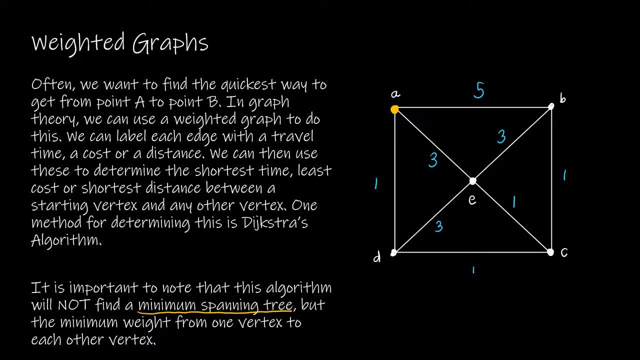 spanning tree is yet We're going to learn that in a little bit, So perhaps that's not confusing to you. If you've studied minimum spanning trees, that is a tree that's going to have some beginning vertex like A and then the cheapest path, or